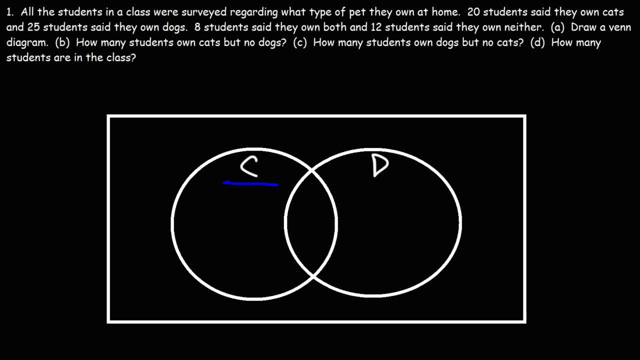 And for the second circle, this is going to represent the number of students who own dogs. Now, in this overlapping region, that represents the students who own cats And that represents the students who own both cats and dogs And that was given to us in the problem. 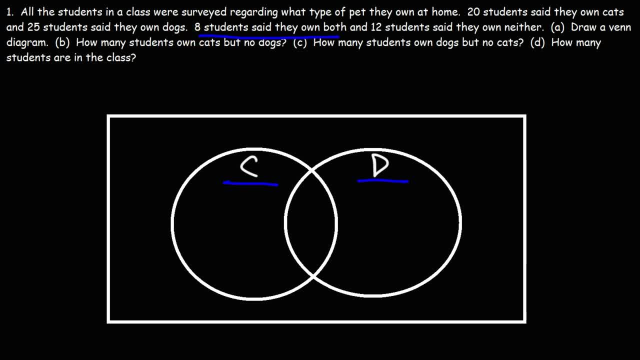 8 students said they own both. So what that means is we can put 8 in this region here. Now what about Part B? How many students own cats but no dogs? So how many students own cats only? We have a total of 20 students who own cats. 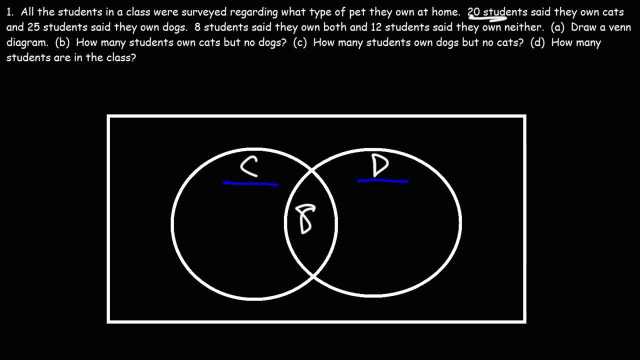 So this includes the 8 who own cats And this includes the students who own both. So to get those who own cats only, we need to subtract 20 by 8. And that's going to give us 12. So we have 12 students who own cats. 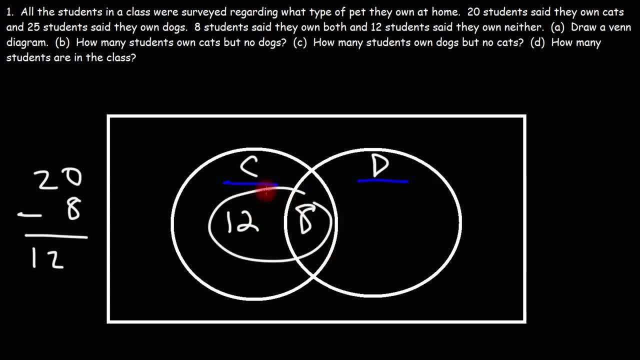 8 own cats and dogs. So we have a total of 20 students who own cats. Now what about Part C? How many students own dogs but no cats? So we have a total of 25 students who own dogs. 8 own both cats and dogs. 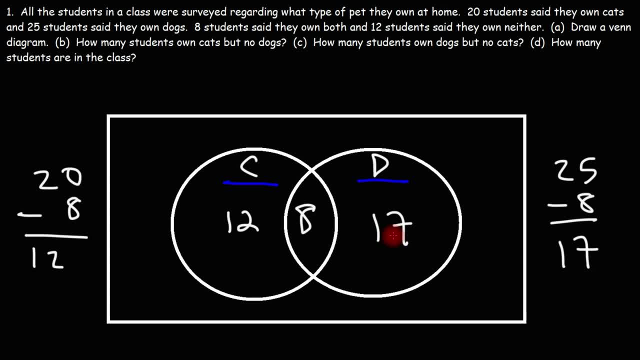 So the difference is 17.. 17 students own dogs only, Or dogs and no cats. Now we have 12 students who own neither cats nor dogs, So we can put that on the outside of the Venn diagram. So now how many students are in the class? 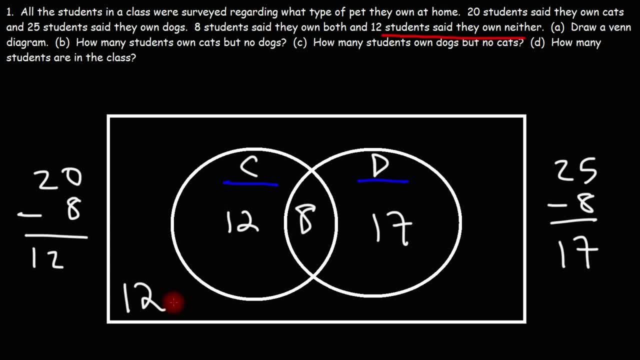 How many students are in the class. How can we get the answer for Part D? There's two ways we can do this. One is when we have the Venn diagram all filled out and completed. The other way involves getting the answer without using the Venn diagram, with the information that we had in the beginning. 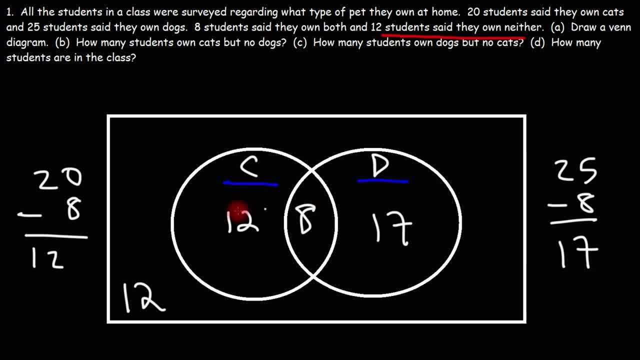 So let's start with the first way. All we need to do is add up the four numbers that we have here, So we have 12 students who own cats, only 17 only own dogs, 8 own both, 12 own neither. 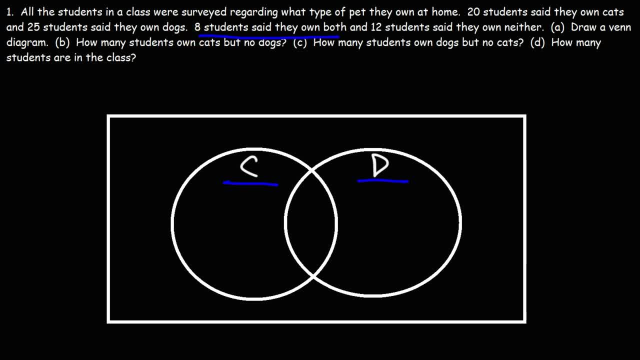 8 students said they own both. So what that means is we can put 8 in this region here. Now what about Part B? How many students own cats but no dogs? So how many students own cats only? We have a total of 20 students who own cats. 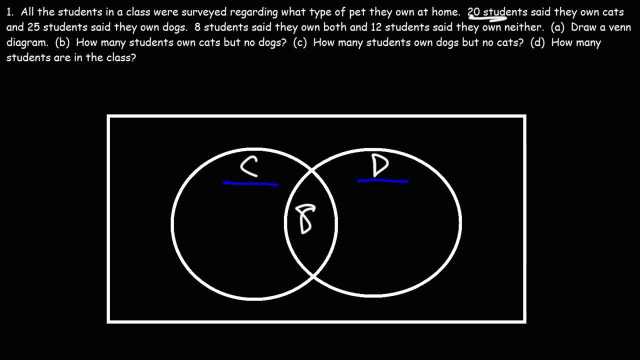 So this includes the 8 who own cats And this includes the students who own both. So to get those who own cats only, we need to subtract 20 by 8. And that's going to give us 12. So we have 12 students who own cats. 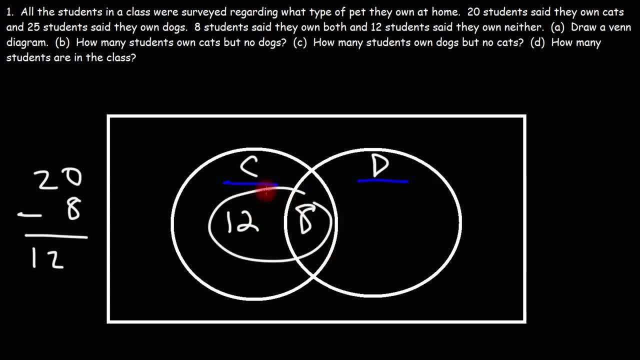 8 own cats and dogs. So we have a total of 20 students who own cats. Now what about Part C? How many students own dogs but no cats? So we have a total of 25 students who own dogs. 8 own both cats and dogs. 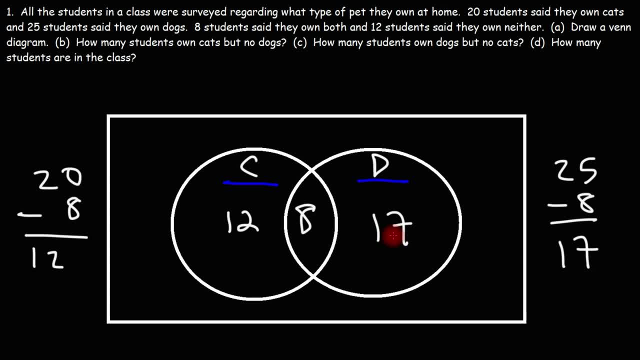 So the difference is 17.. 17 students own dogs only, Or dogs and no cats. Now we have 12 students who own neither cats nor dogs, So we can put that on the outside of the Venn diagram. So now how many students are in the class? 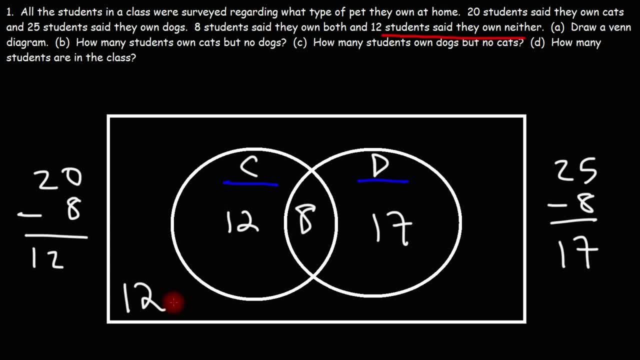 How many students are in the class. How can we get the answer for Part D? There's two ways we can do this. One is when we have the Venn diagram all filled out and completed. The other way involves getting the answer without using the Venn diagram, with the information that we had in the beginning. 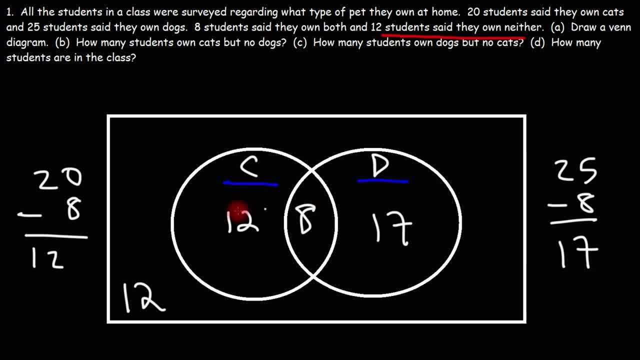 So let's start with the first way. All we need to do is add up the four numbers that we have here, So we have 12 students who own cats, only 17 only own dogs, 8 own both, 12 own neither. 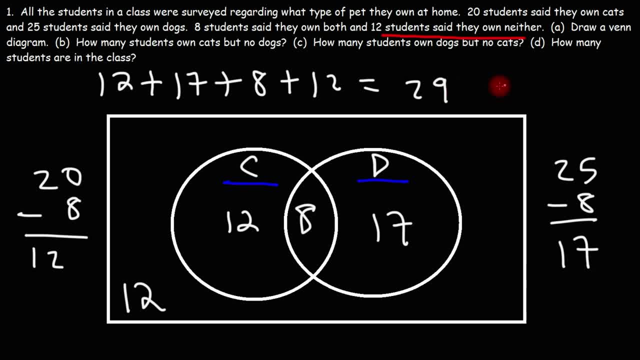 12 plus 17 is 29.. 8 plus 12 is 20.. 29 plus 20 is 49. So we have a total of 49 students who were surveyed in this class And since all the students in the class were surveyed, 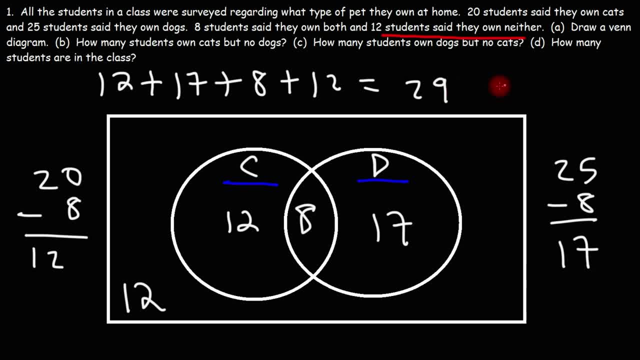 12 plus 17 is 29.. 8 plus 12 is 20.. 29 plus 20 is 49. So we have a total of 49 students who were surveyed in this class And since all the students in the class were surveyed, 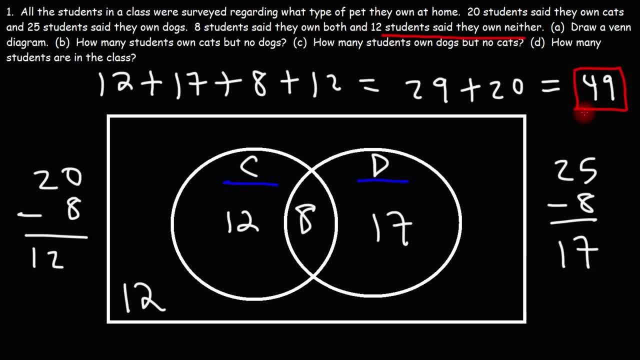 there are 49 students in this class. Now, to do it the second way, without the Venn diagram, using the information that we started with, we're going to add up the number of students who own cats and dogs, So we have 20 students who own cats. 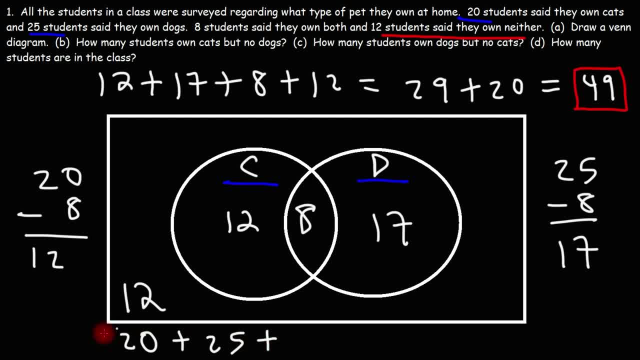 25 own dogs. But now both of these numbers include the students who own cats and dogs, That is, the students who own both, And since we've counted it twice, we need to subtract it once, Because we only want to include this number once. 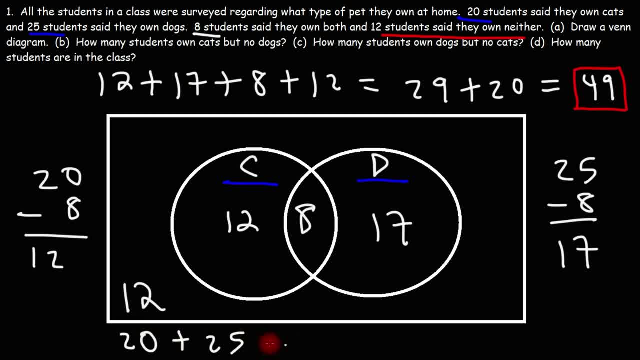 So, since we already included it twice in both these numbers, we're going to subtract this by 8 once, so that we've counted this quantity only one time. And then, finally, we need to add the number of students who own neither, which is 12.. 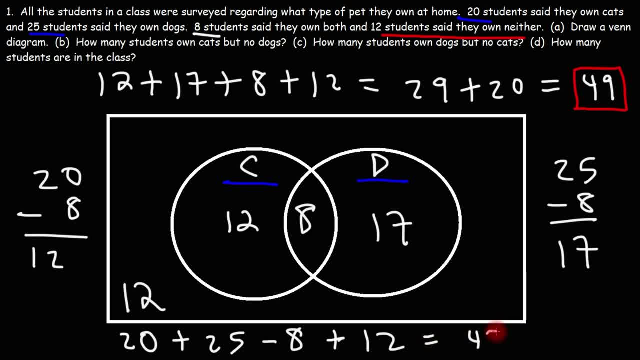 So 20 plus 25 is 45. And then negative 8 plus 12,, that's positive 4.. And this will give us the same number of 49 students who are in this class. So those are two ways in which you can get the final answer. 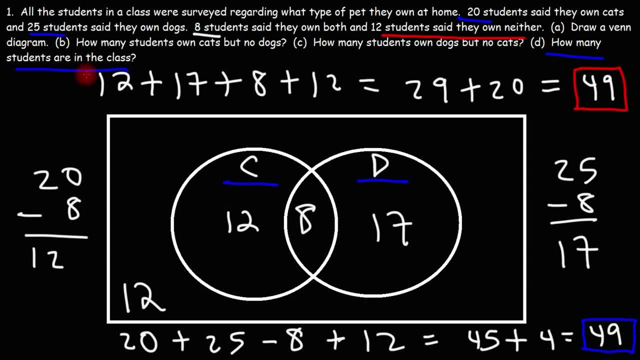 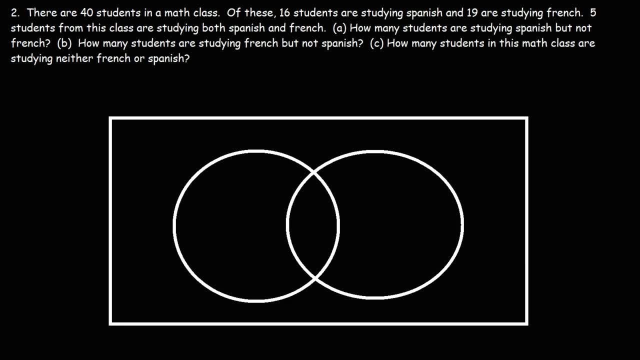 if you have to get the total sum of everyone involved in the survey. Now let's work on a slightly different problem. In this problem we're given the total number of students in the class. We didn't have that information in the last problem. 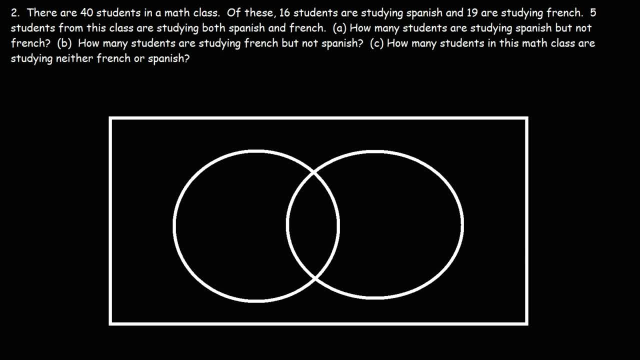 However, in this problem, we don't know how many students are studying neither Spanish or French. In the last problem, we had the number of students who own neither dogs or cats. So that's the difference between these two problems. So go ahead and feel free to pause the video. 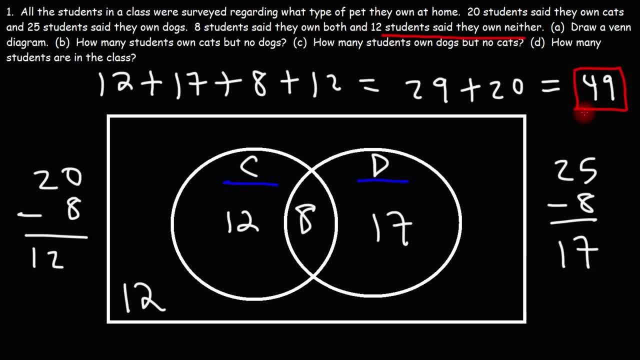 there are 49 students in this class. Now, to do it the second way, without the Venn diagram, using the information that we started with, we're going to add up the number of students who own cats and dogs, So we have 20 students who own cats. 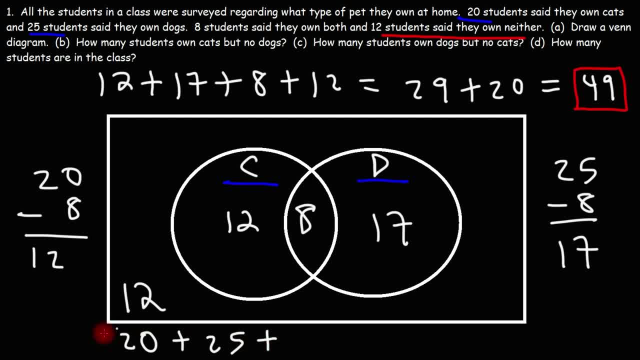 25 own dogs. But now both of these numbers include the students who own cats and dogs, That is, the students who own both, And since we've counted it twice, we need to subtract it once, Because we only want to include this number once. 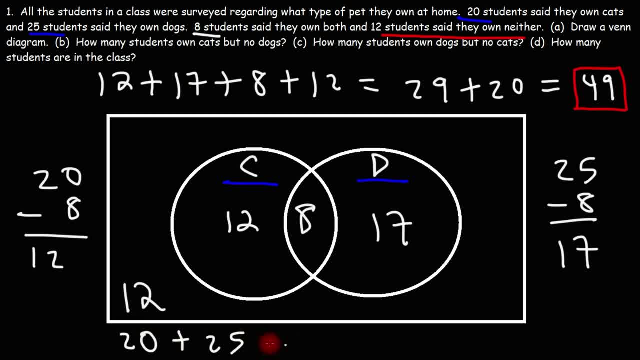 So, since we already included it twice in both these numbers, we're going to subtract this by 8 once, so that we've counted this quantity only one time. And then, finally, we need to add the number of students who own neither, which is 12.. 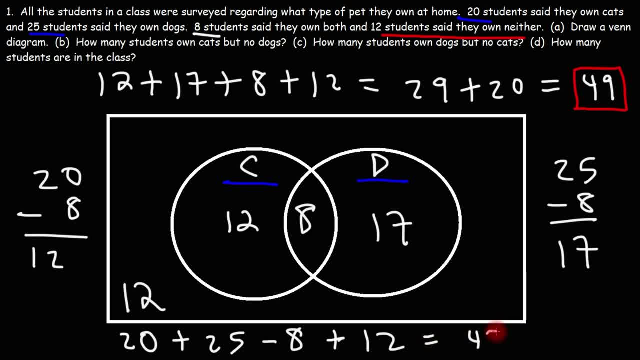 So 20 plus 25 is 45. And then negative 8 plus 12,, that's positive 4.. And this will give us the same number of 49 students who are in this class. So those are two ways in which you can get the final answer. 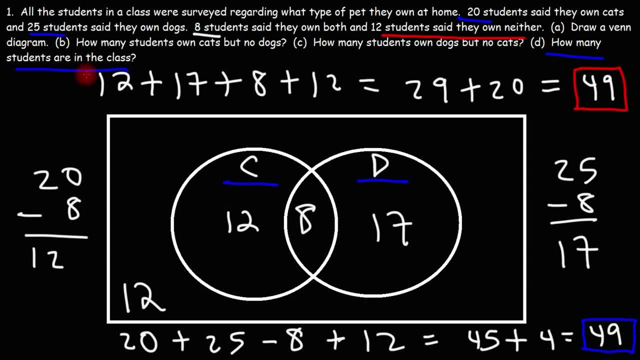 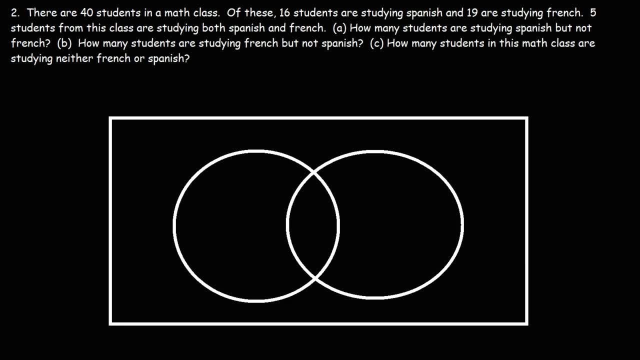 if you have to get the total sum of everyone involved in the survey. Now let's work on a slightly different problem. In this problem we're given the total number of students in the class. We didn't have that information in the last problem. 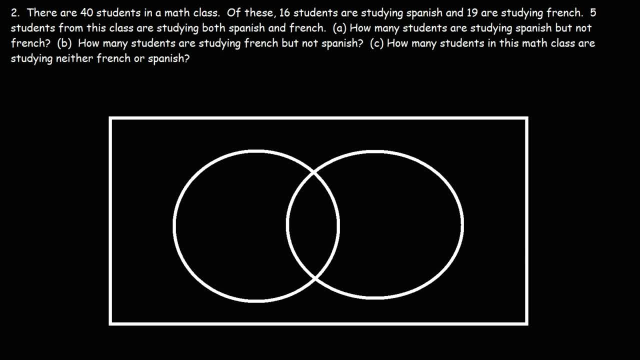 However, in this problem, we don't know how many students are studying neither Spanish or French. In the last problem, we had the number of students who own neither dogs or cats. So that's the difference between these two problems. So go ahead and feel free to pause the video. 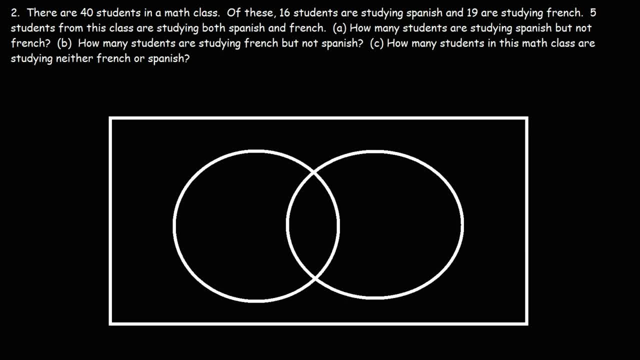 and try this problem. So there are 40 students in a math class. Of these, 16 students are studying Spanish and 19 are studying French. Five students from this class are studying both Spanish and French, Part 8.. How many students are studying Spanish but not French? 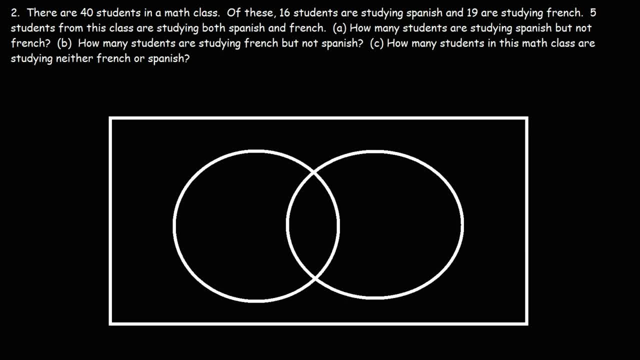 and try this problem. So there are 40 students in a math class. Of these, 16 students are studying Spanish and 19 are studying French. Five students from this class are studying both Spanish and French, Part 8.. How many students are studying Spanish but not French? 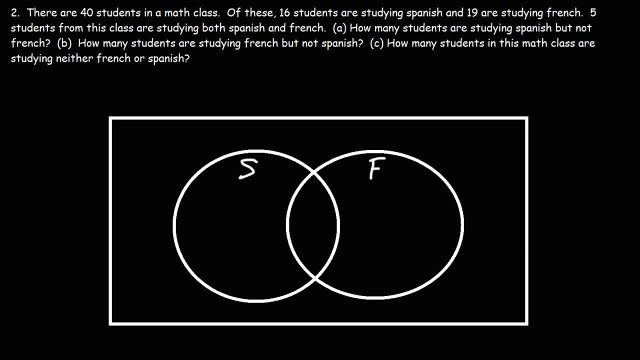 So let's put S for Spanish, F for French. Now the first thing I'd like to do, just like in the last problem, is I'd like to put the number of students who are studying in both categories, And that's five. 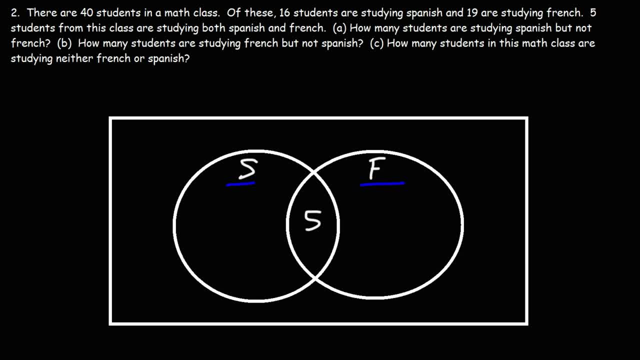 So let's put that in the middle. So now, how many students are studying Spanish but not French? So we have a total of 16 students who are studying Spanish. Five of them are studying both Spanish and French, though the difference will give us those who are studying only Spanish but not French. 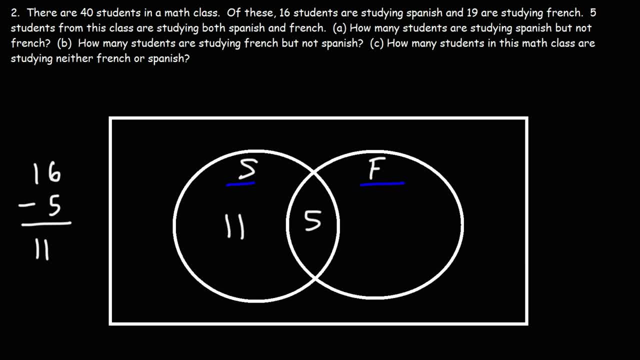 And that's going to be 11.. Part B: How many students are studying French but not Spanish? So we have a total of 19 who are studying French, Five are studying both, So only 14 are studying French but not Spanish. 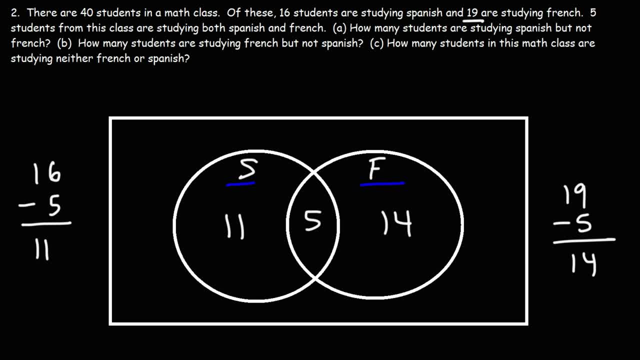 Now, how do we find out in Part C how many students in this math class are studying neither French or Spanish? So, basically, how can we find the number that belongs outside of the Venn diagram? Now remember how we got our total in the last problem. 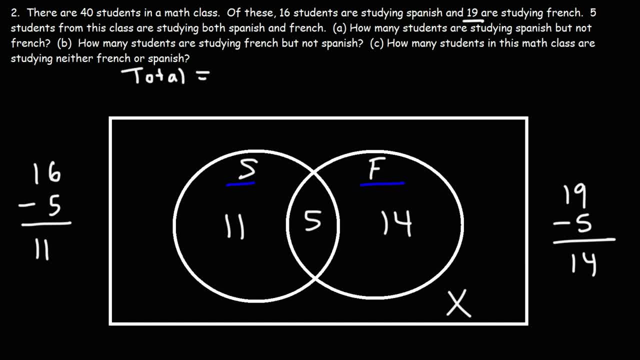 The total number of students- this is the first method used in the Venn diagram- is basically the sum of all of these numbers, So it's the 11 students studying Spanish only, plus the 14 students studying French but not Spanish. 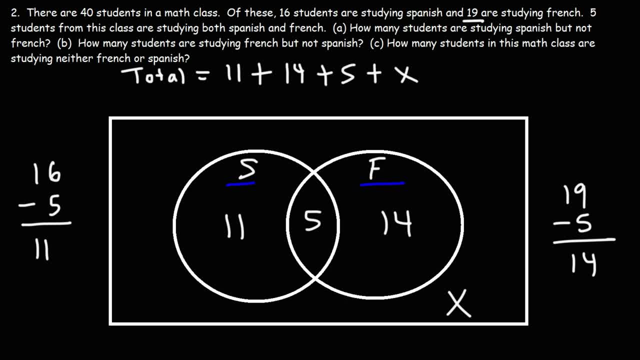 the 5 who are studying both and the number who are studying neither, which is what we're looking for. So that's x And we have the total. The total is: we've got 40 students in the class, So we have 40 is equal to 11,. 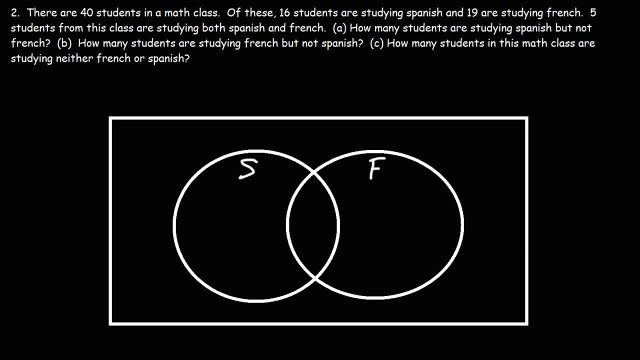 So let's put S for Spanish, F for French. Now the first thing I'd like to do, just like in the last problem, is I'd like to put the number of students who are studying in both categories, And that's five. 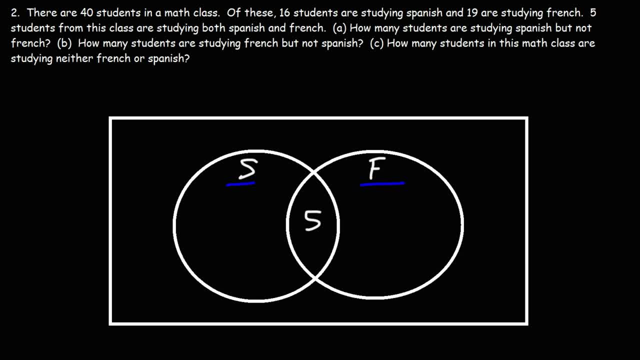 So let's put that in the middle. So now, how many students are studying Spanish but not French? So we have a total of 16 students who are studying Spanish. Five of them are studying both Spanish and French, though the difference will give us those who are studying only Spanish but not French. 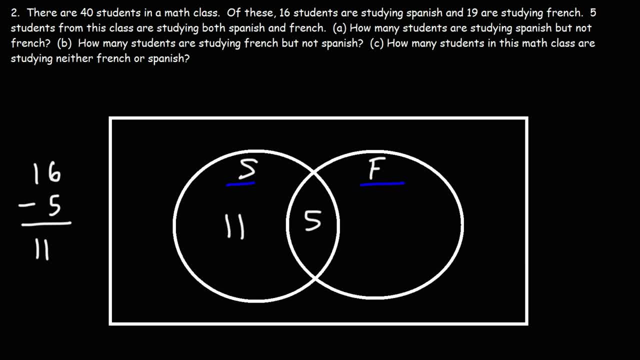 And that's going to be 11.. Part B: How many students are studying French but not Spanish? So we have a total of 19 who are studying French, Five are studying both, So only 14 are studying French but not Spanish. 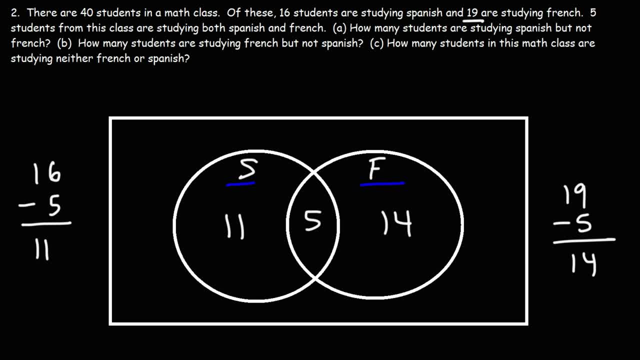 Now, how do we find out in Part C how many students in this math class are studying neither French or Spanish? So, basically, how can we find the number that belongs outside of the Venn diagram? Now remember how we got our total in the last problem. 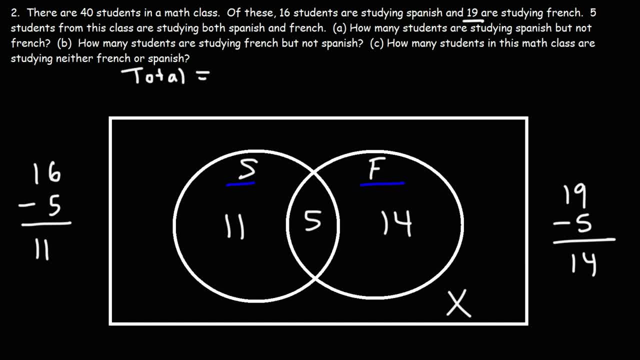 The total number of students- this is the first method used in the Venn diagram- is basically the sum of all of these numbers, So it's the 11 students studying Spanish only, plus the 14 students studying French but not Spanish. 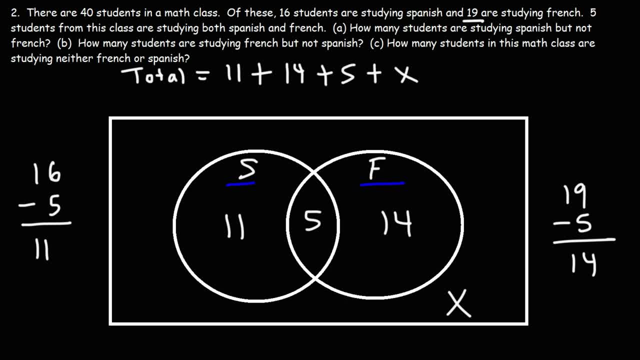 the 5 who are studying both and the number who are studying neither, which is what we're looking for. So that's x And we have the total. The total is: we've got 40 students in the class, So we have 40 is equal to 11,. 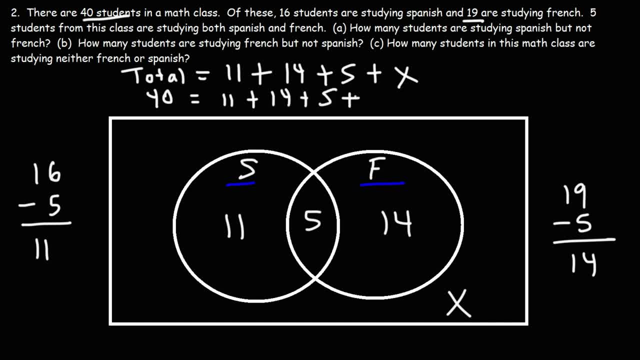 plus 14, plus 5, plus x. So now all we've got to do is solve for x. So let's go ahead and combine like terms: 11 plus 14, that's going to be 25.. And then 25 plus 5,. 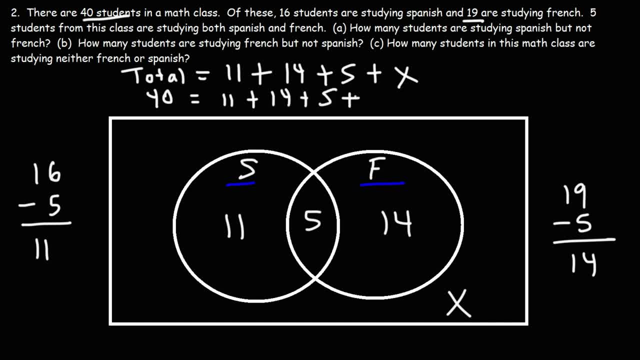 plus 14, plus 5, plus x. So now all we've got to do is solve for x. So let's go ahead and combine like terms: 11 plus 14, that's going to be 25.. And then 25 plus 5,. 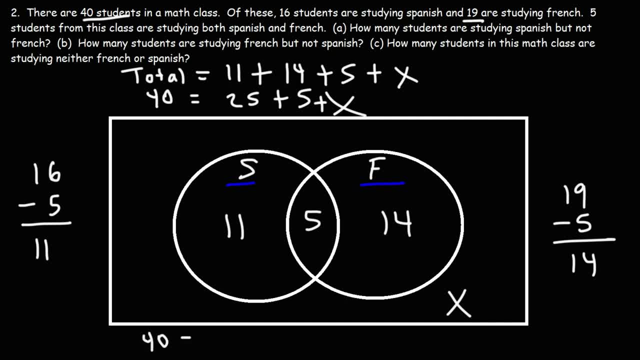 that's 30, so I'm going to write that here. So we have: 40 is equal to 30, plus x. Now we need to subtract both sides by 30. So we're going to have: 40 minus 30 is equal to x. 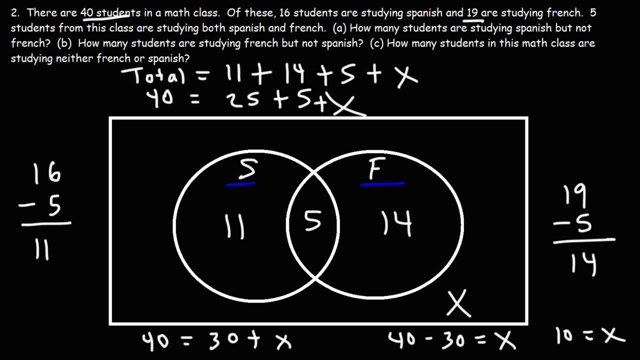 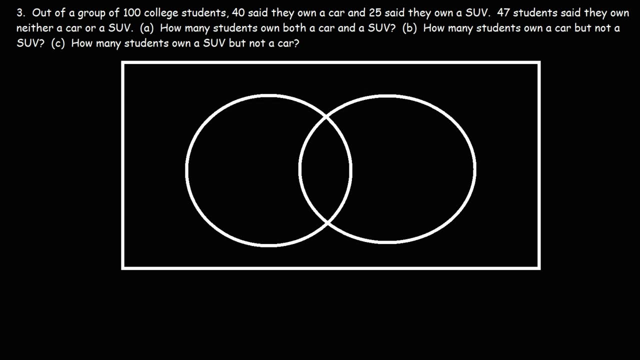 and 40 minus 30 is 10.. So we have 10 students who belong here who are studying neither French nor Spanish. So that's it for this problem. Now let's move on to the third problem Out of a group of 100 college students. 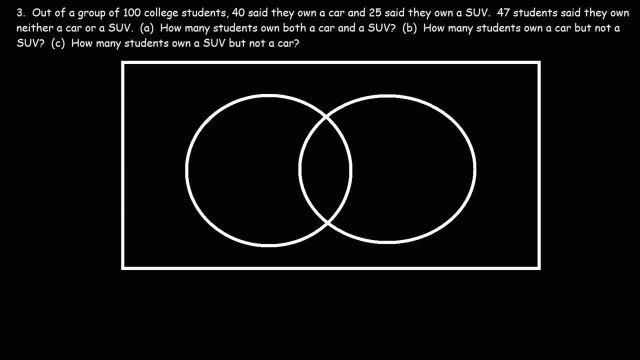 40 said they own a car and 25 said they own an SUV. 47 students said they own neither a car or SUV. So how many students own both a car and an SUV? Now let's recap what we've done so far. 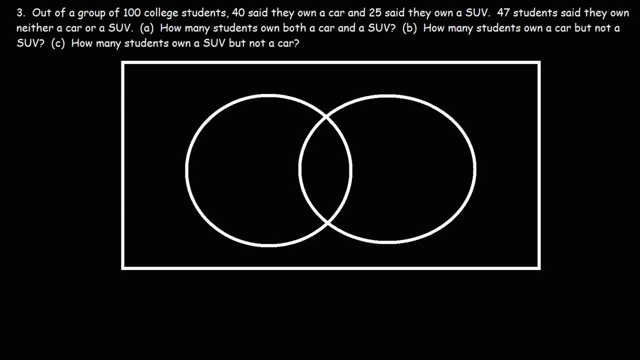 So in problem one we needed to calculate the total number of students who own cats and dogs. In problem two, we didn't know the neither part. We didn't know the number of students who took neither Spanish or French, So that was the missing element. 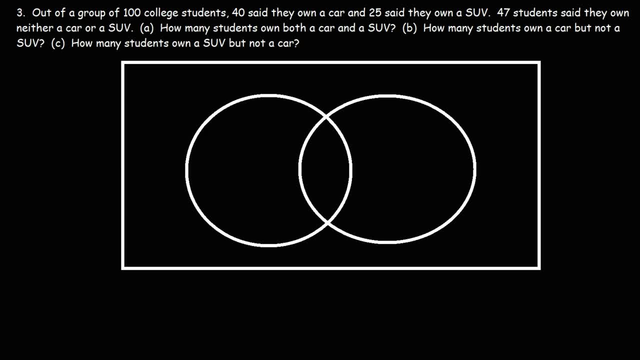 In problem three, the missing element is both: We don't know how many students own both a car and an SUV, And so those are the three types of variations that we can have with this two-category-then-diagram problem. So how can we calculate? 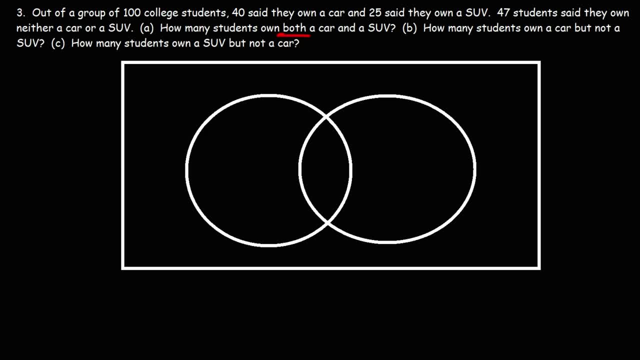 the both part. It helps to write a formula. So let's put C for cars, S for SUV, B for both, so that's the number that goes in here and N for neither. Now using method two to get the total. 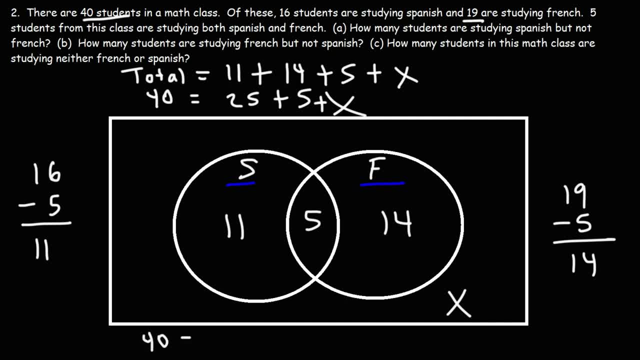 that's 30, so I'm going to write that here. So we have: 40 is equal to 30, plus x. Now we need to subtract both sides by 30. So we're going to have: 40 minus 30 is equal to x. 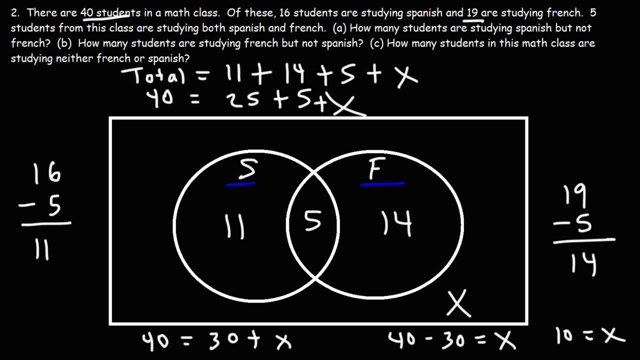 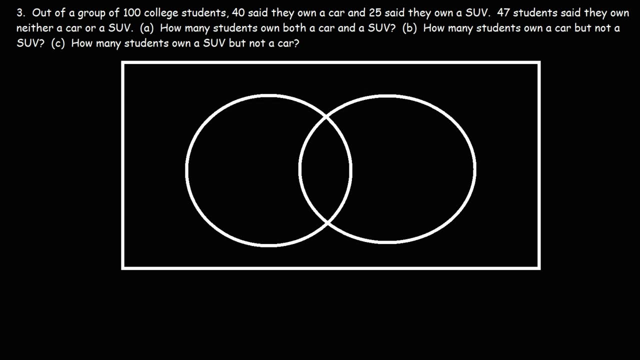 and 40 minus 30 is 10.. So we have 10 students who belong here who are studying neither French nor Spanish. So that's it for this problem. Now let's move on to the third problem Out of a group of 100 college students. 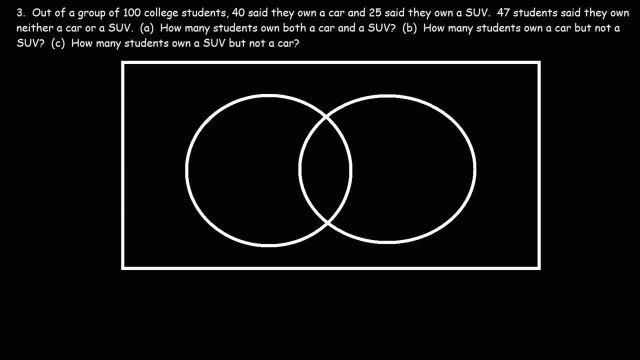 40 said they own a car and 25 said they own an SUV. 47 students said they own neither a car or SUV. So how many students own both a car and an SUV? Now let's recap what we've done so far. 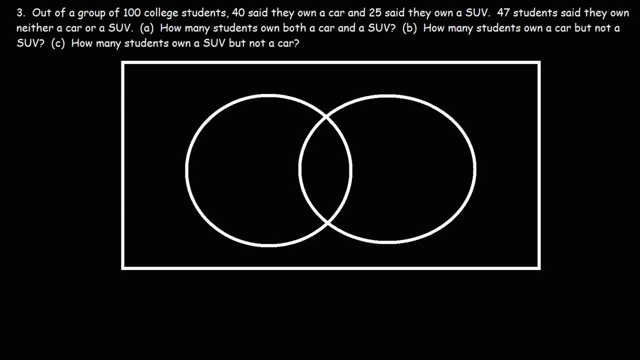 So in problem one we needed to calculate the total number of students who own cats and dogs. In problem two, we didn't know the neither part. We didn't know the number of students who took neither Spanish or French, So that was the missing element. 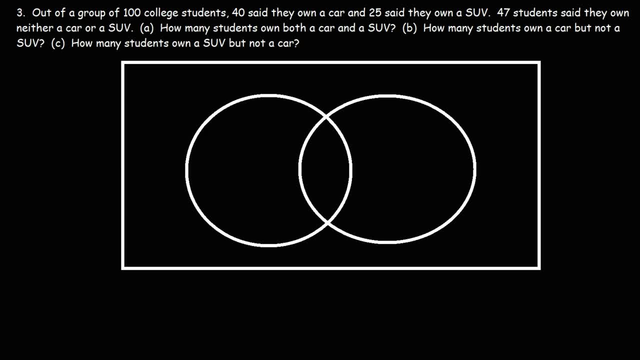 In problem three, the missing element is both: We don't know how many students own both a car and an SUV, And so those are the three types of variations that we can have with this two-category-then-diagram problem. So how can we calculate? 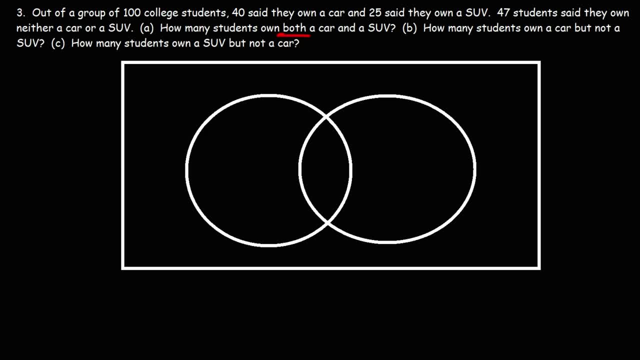 the both part. It helps to write a formula. So let's put C for cars, S for SUV, B for both, so that's the number that goes in here and N for neither. Now using method two to get the total. 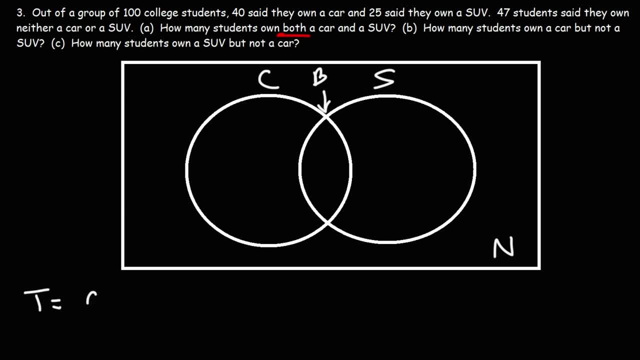 it would be all the students who own cars, which would be this entire circle, plus all the students who own SUVs, which would be this entire circle. But doing it this way, we counted this part twice, so we would have to subtract by B. 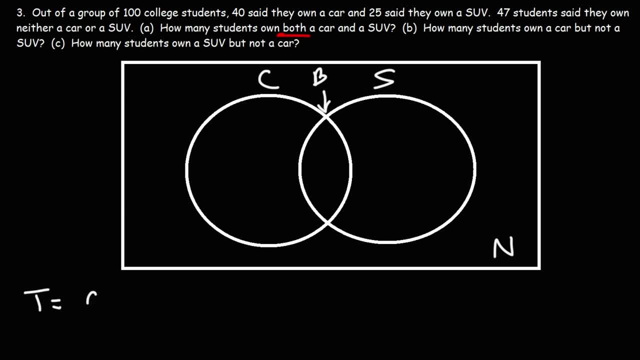 it would be all the students who own cars, which would be this entire circle, plus all the students who own SUVs, which would be this entire circle. But doing it this way, we counted this part twice, so we would have to subtract by B. 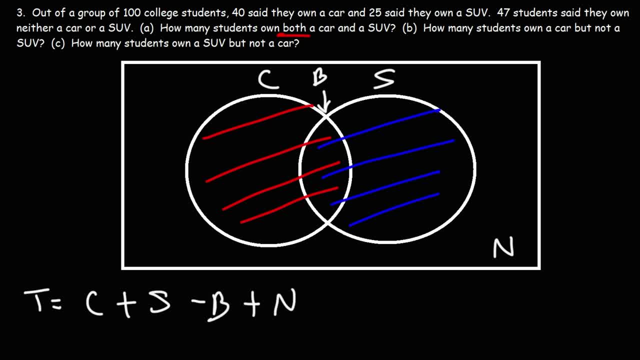 and then add N, So that would be method one. So it's C plus S minus B plus N. Method two to calculate the total would be the students who own cars. only That would be C minus B. C represents all the students who own cars. 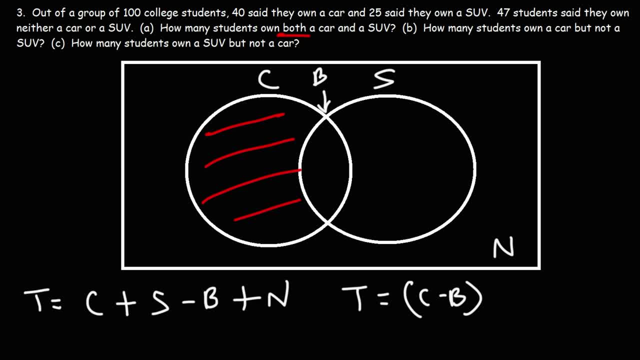 So if you subtract those who own both cars and SUVs, you get those who own cars only. Now to get those who own SUVs only, it's S minus B. So that would represent this part here. Now we need to add the middle part. 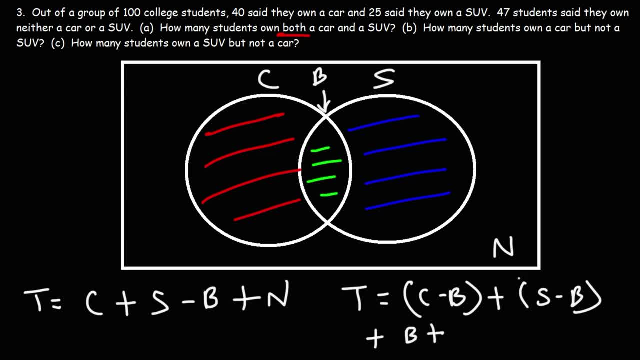 So we would have plus B and then those who own neither plus N. But notice that the equation on the right simplifies to the equation on the left. If you cancel negative B and B, you get C plus S minus B plus N. 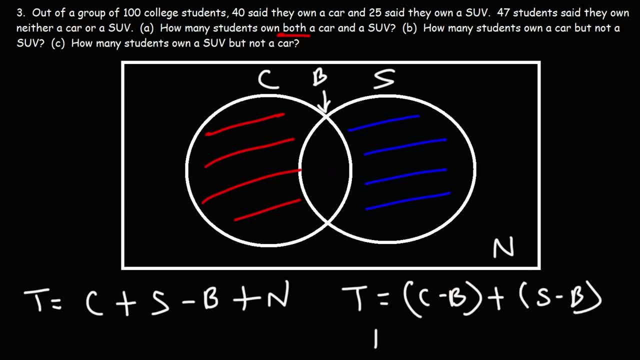 So both equations lead to the same result. So let's go ahead and use this equation to calculate B. So the total number of students is 100 college students. Now we know that 40 said they own a car, 25 said they own an SUV. 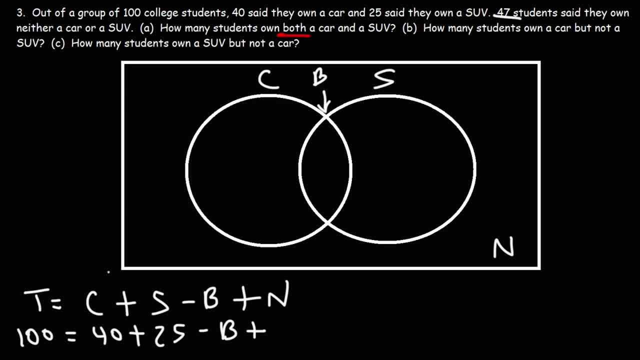 Our goal is to calculate B and 47 said they own neither. So let's put this here: N is 47.. So now let's do some algebra. Let's combine like terms: 40 plus 25,, that's 65.. 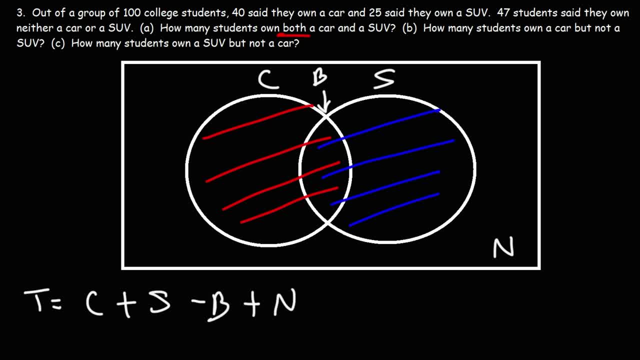 and then add N, So that would be method one. So it's C plus S minus B plus N. Method two to calculate the total would be the students who own cars. only That would be C minus B. C represents all the students who own cars. 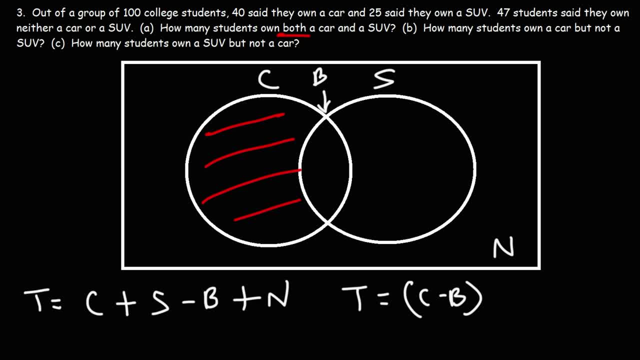 So if you subtract those who own both cars and SUVs, you get those who own cars only. Now to get those who own SUVs only, it's S minus B. So that would represent this part here. Now we need to add the middle part. 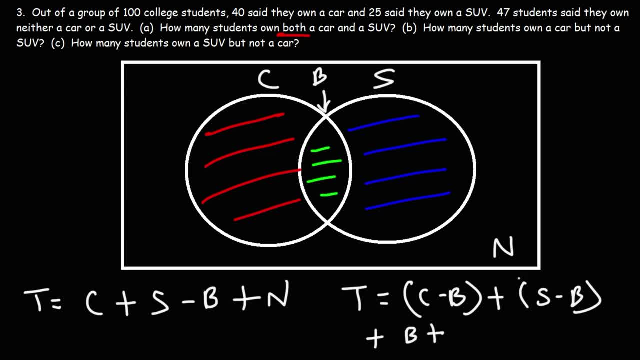 So we would have plus B and then those who own neither plus N. But notice that the equation on the right simplifies to the equation on the left. If you cancel negative B and B, you get C plus S minus B plus N. 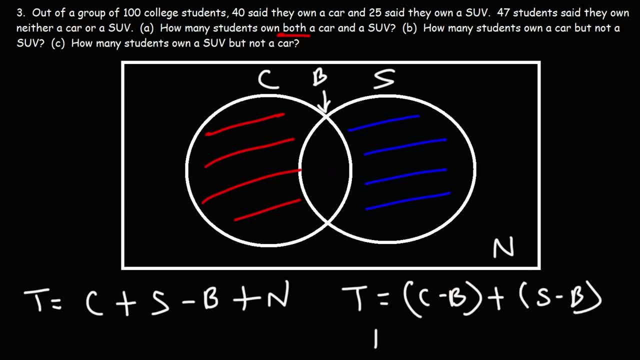 So both equations lead to the same result. So let's go ahead and use this equation to calculate B. So the total number of students is 100 college students. Now we know that 40 said they own a car, 25 said they own an SUV. 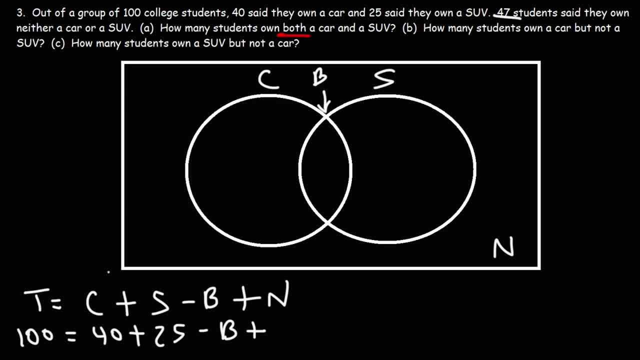 Our goal is to calculate B and 47 said they own neither. So let's put this here: N is 47.. So now let's do some algebra. Let's combine like terms: 40 plus 25,, that's 65.. 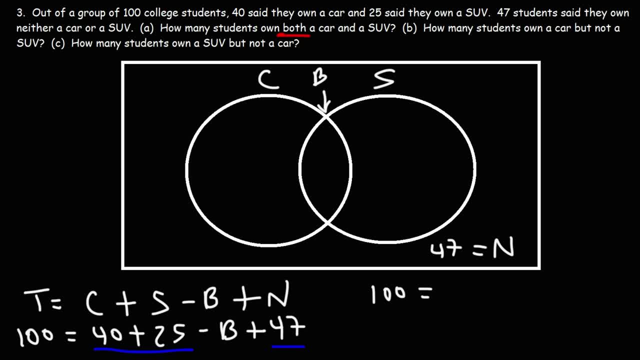 And 65 plus 45, I mean 65 plus 47, rather, that is 112.. So 112 minus what number is 100?? B has to be 12.. If you want to show your work, subtract both sides by 112.. 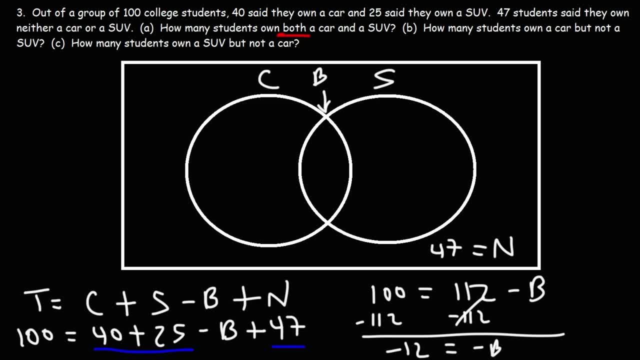 You're going to get negative. 12 is equal to negative B. Multiply both sides by negative 1, you get B is 12.. So we have 12 students who own both a car and an SUV. So that's it for part A.